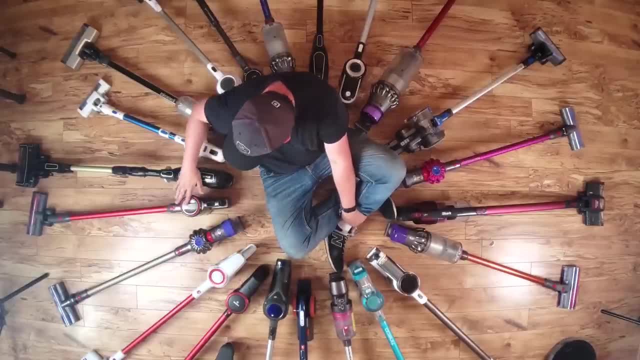 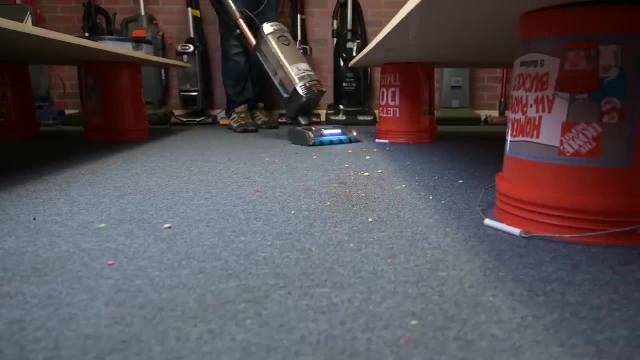 theoretically choose any one that I want at any price. So in this video I'll take you behind the scenes and show you which ones I actually use. Before I answer that, though, I should point out a few things. I actually use about seven vacuums on a regular basis, both at home and at the. 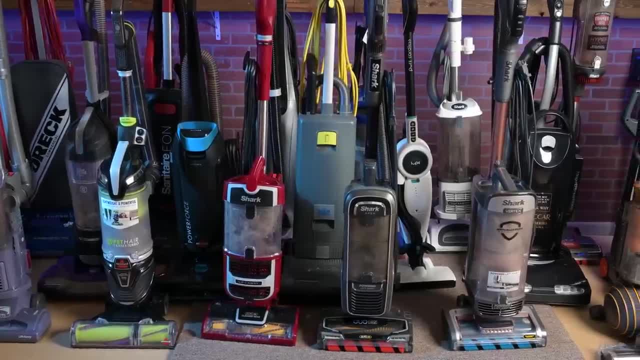 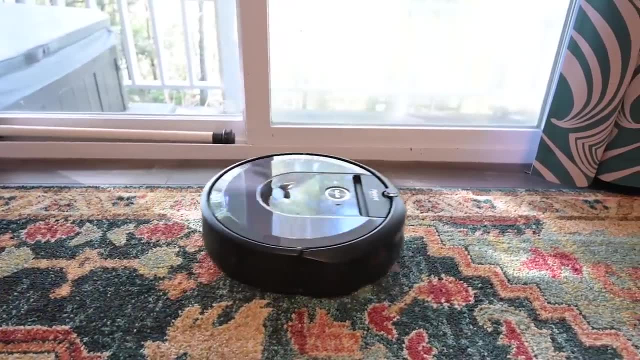 Vacuum Wars studio, Because I have so many to choose from. I find that I use specific vacuums for specific jobs, which we'll see in a moment. I also wanted to mention that of these seven or so vacuums. they change all the time as new ones come out, and I'll mention a few things about that as 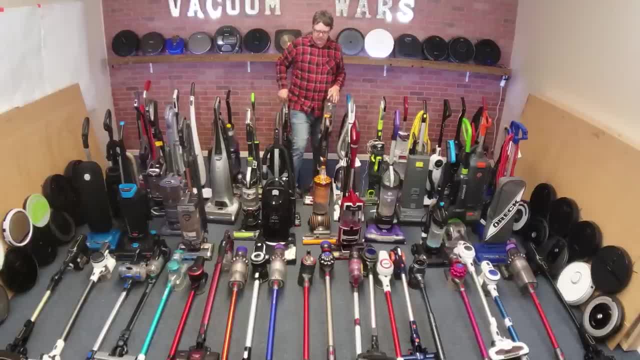 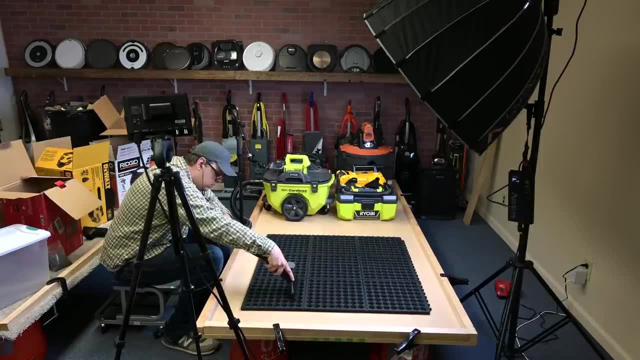 we progress as well. So links in the description to everything I'll mention. and let's get started. I'm going to start off by talking about which vacuum I use at Vacuum Wars studios, where I'm always doing some kind of messy test with vacuums, and 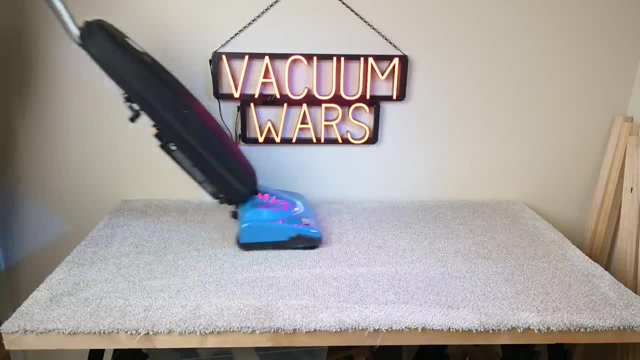 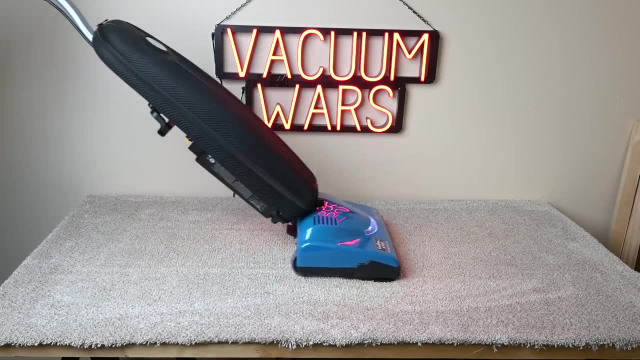 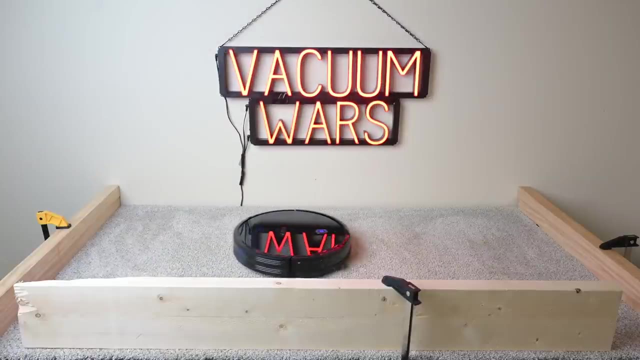 robot vacuums. One vacuum that's seen a lot of use at the studio since I bought it almost a year ago is the Recar Superlite Cordless R10CV. I use this one for resetting my deep clean test, where I embed exactly 100 grams of sand into medium pile carpet to see how good vacuums are. 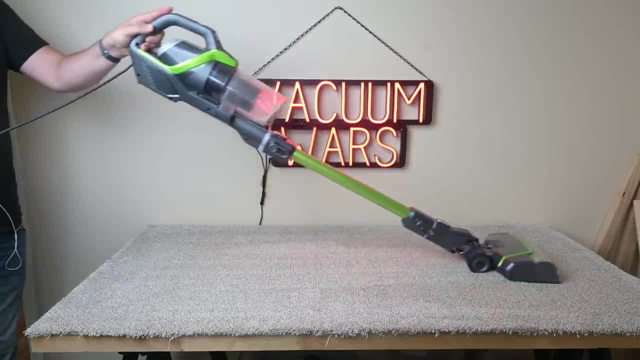 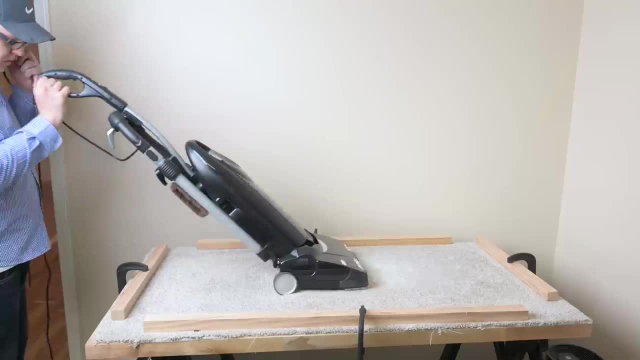 at getting deep down debris in carpets. This is a test where it's absolutely critical that I get all the sand out of the carpet and I don't want to get any sand in the carpet, So I'm going to from the previous test to make sure I have accurate results. Recar corded vacuums are 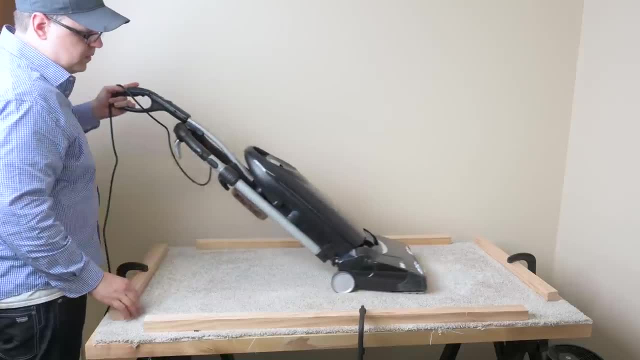 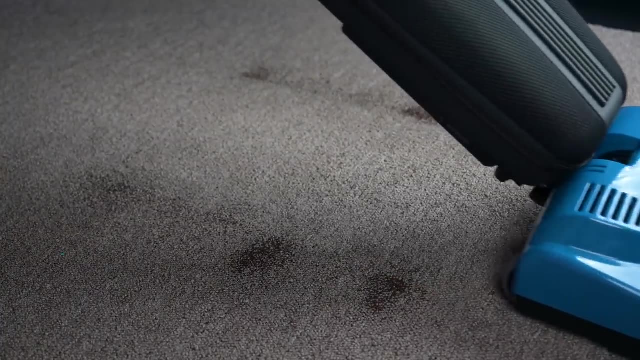 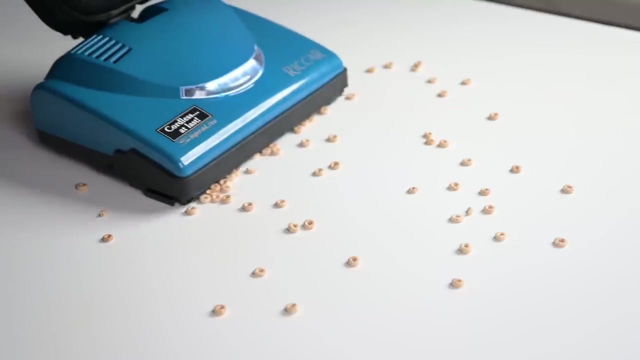 expensive but amazing with carpet agitation, and they have a ton of power. When I tested their cordless version, the R10CV, I was pretty skeptical, but it has the same great agitation as their corded vacuums and it has a ton of power for a cordless. It still has its limitations, to be sure. 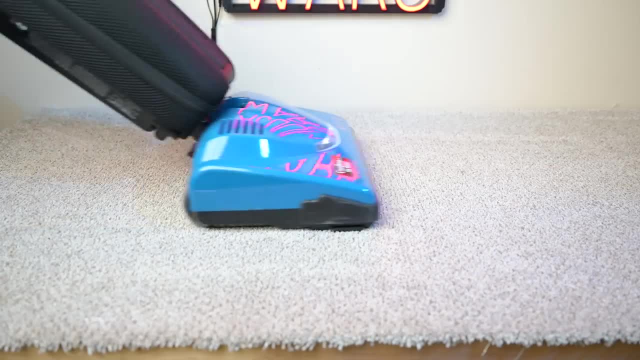 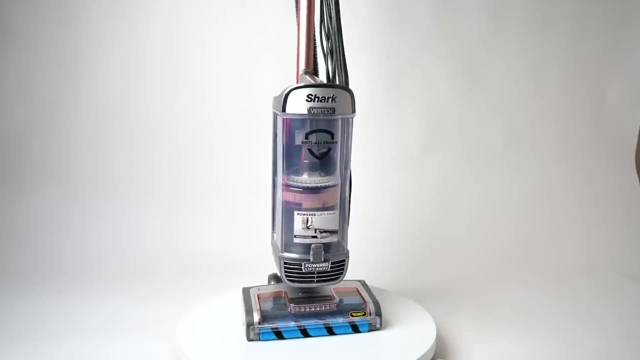 and I don't use it for much else besides this, but it has become my go-to vacuum for when I need carpet cleaned and I need to be out of the car. So I'm going to start with the Recar Superlite Vacuum War Studio and I'm absolutely sure it did the job. I also used the new Shark Vertex at the 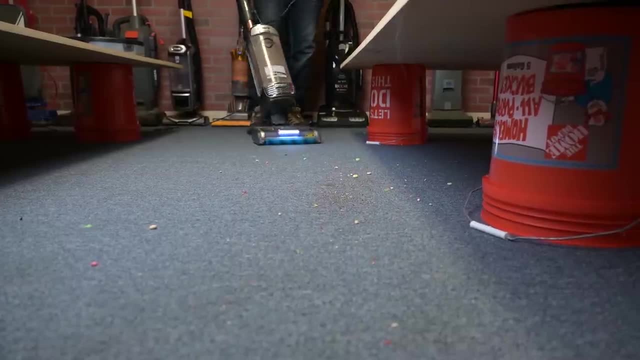 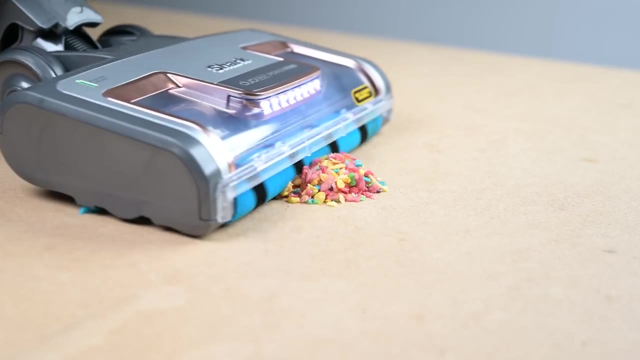 Vacuum War Studio, mostly for picking up the big messes that other vacuums leave behind. I used to use the Shark Apex Zero M for this purpose, but since the Vertex came out and after our review of the Vertex I realized it was basically the slightly better version of the Apex I have. 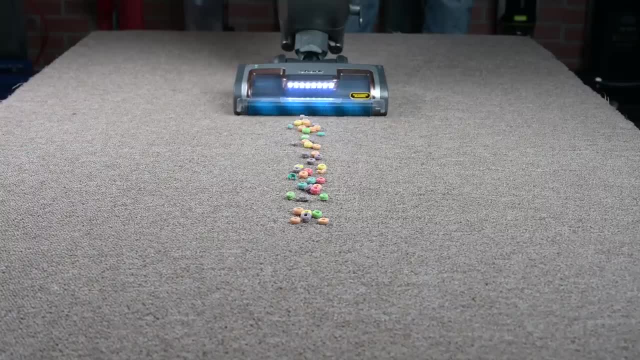 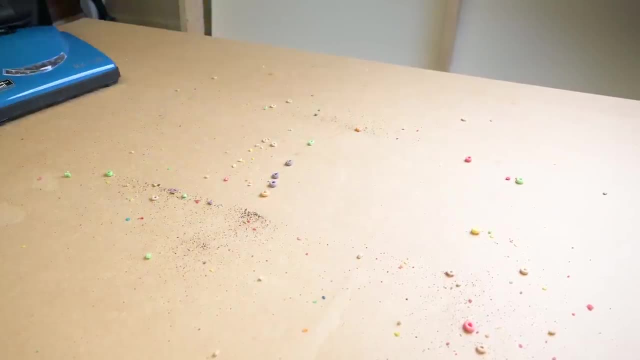 retired my Shark Apex. I actually gave it to my mom and started using the Vertex instead. Anyway, since most vacuums can't pick up everything I throw at them in the various tests, there is inevitably a big mess left behind, at least once or twice a week. The Vertex is the 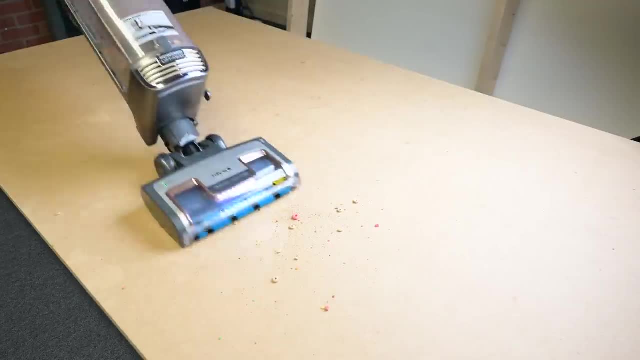 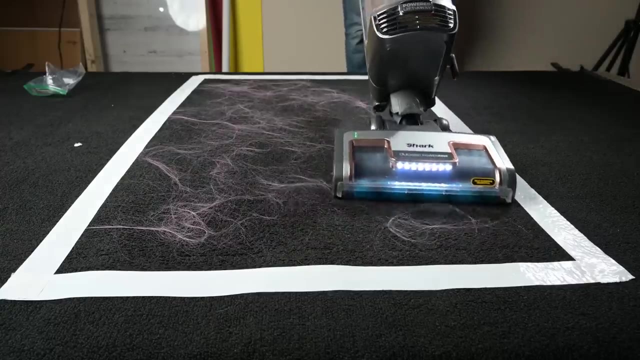 vacuum that I turn to when it has to be picked up. It's the vacuum of last resort. It's the one I turn to when it's too big for anything else. I can also trust it if it's picking up after a major hair tangle test, because it's one of the best at resisting hair tangles as well. I will also. 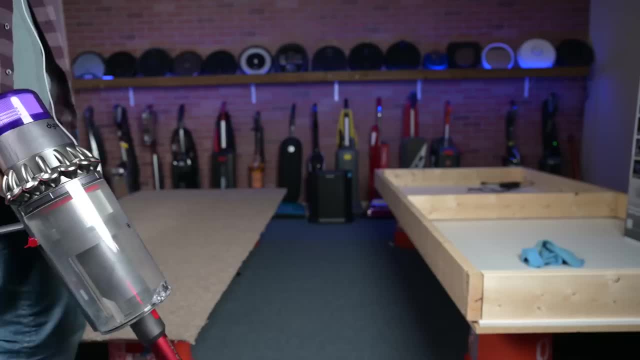 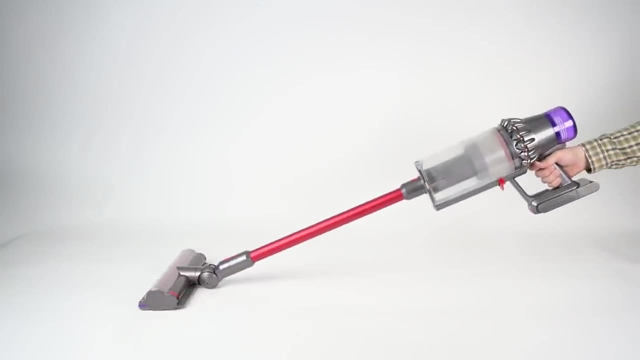 occasionally use it to clean the whole studio, but mostly that job falls to whatever the current best Dyson cordless is, which in this case is the Dyson Apex. I use my Dyson V11 cordless vacuum- a lot like the Vertex actually. In fact I prefer to use the V11. 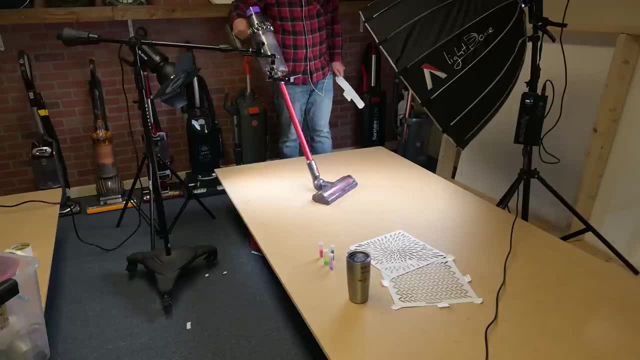 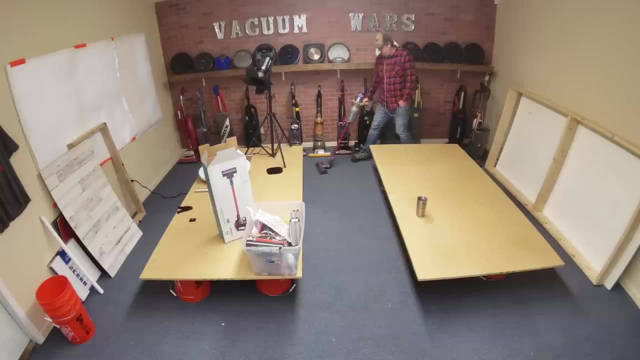 for cleaning up after and resetting the stage if the mess from the previous vacuum isn't too big, because the V11 is cordless and thus more convenient than the Vertex. I also use the V11 to clean the whole studio more often than not, mostly again because it's convenient. it's light. 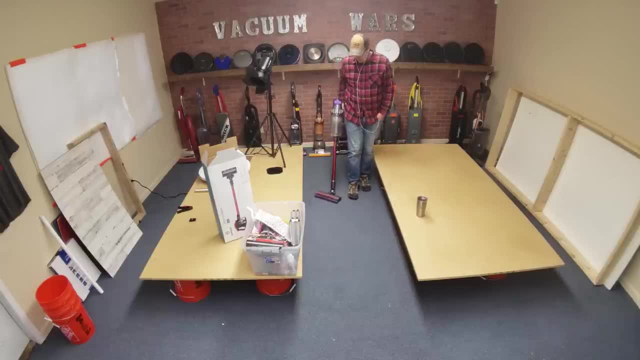 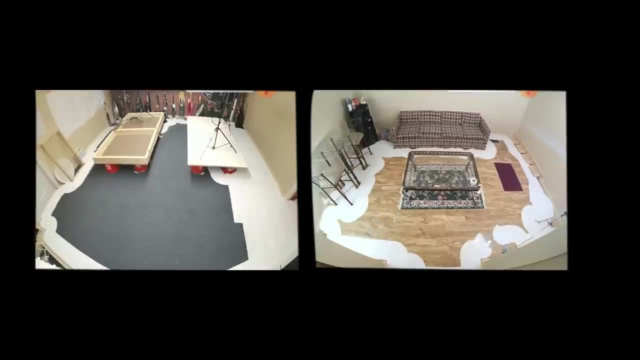 it's cordless, but I really do love using Dyson cordless vacs. I think in general, they are the best in terms of build quality, power and performance. I also use the V11 to clean the studio, in the past, like the Roborock S5, and more recently, the Roborock S5 Max, which I think. 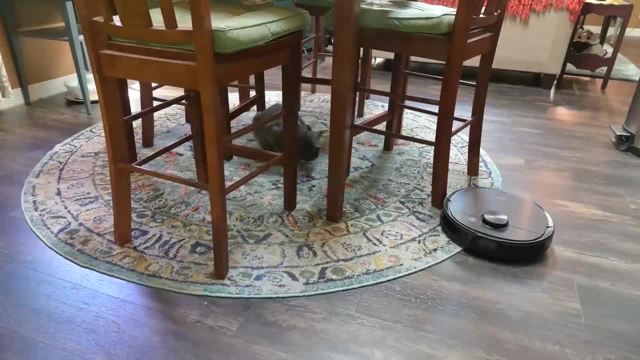 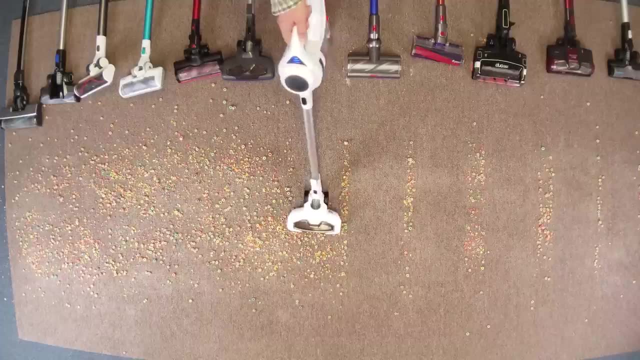 are great all-around robot vacuums, but these days I only use robot vacuums at home, since the studio setup changes too much and I could be in the middle of some large test with stuff all over the floor for some video shoot, so I just find it's better just to vacuum the studio without 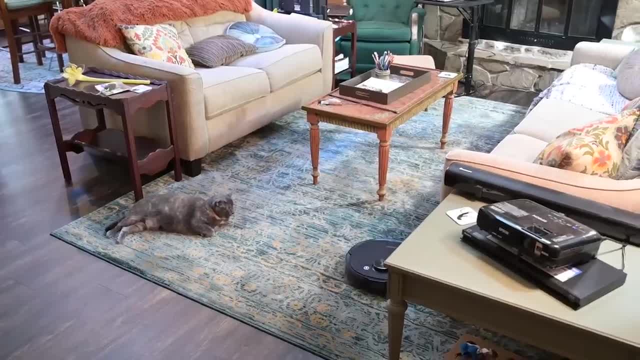 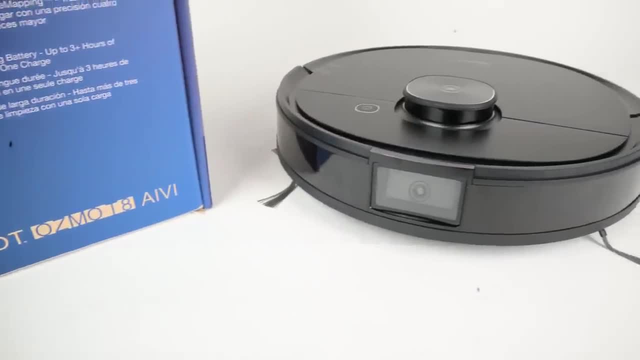 robots. So that brings me to the vacuums I use at my home, and here again there is more than one. I'll start off with the one I've mentioned recently, the Ecovacs T8 AIVI robot vacuum with the auto empty bin. This is currently the top of the line robot vacuum from Ecovacs. 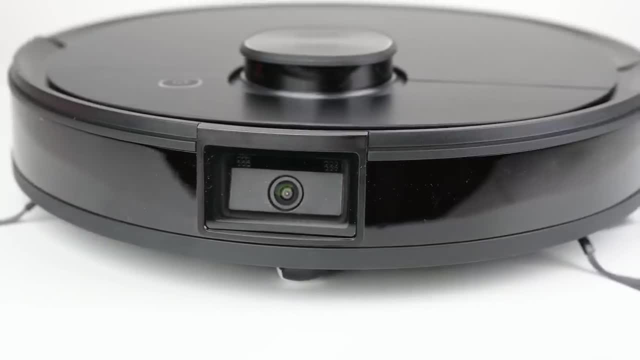 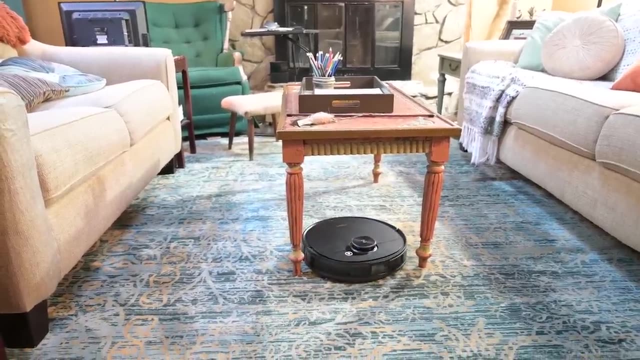 which has all the bells and whistles, including the front mounted camera and AI obstacle avoidance system. We use it on the upstairs level of our house for vacuuming as well as mopping, and it seems like we'll continue to do so until something better comes along, which. 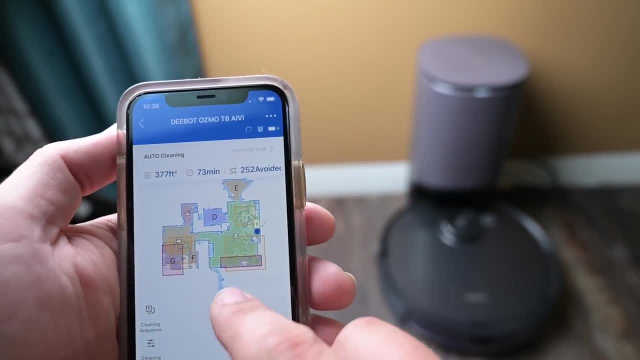 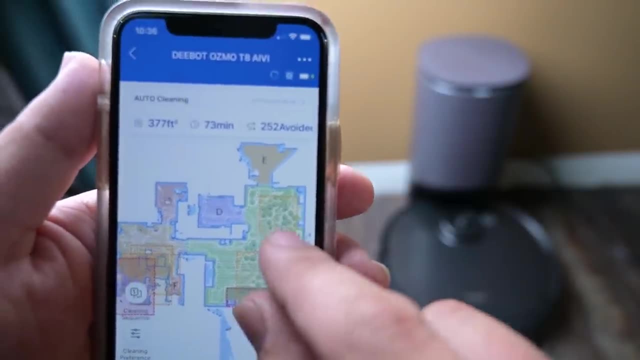 it almost always does. The upstairs has a lot more difficult areas to navigate around, so it's important to have one that we could highly customize the map with, using lots of no go and no mop lines to keep it out of certain areas. One update from that review. 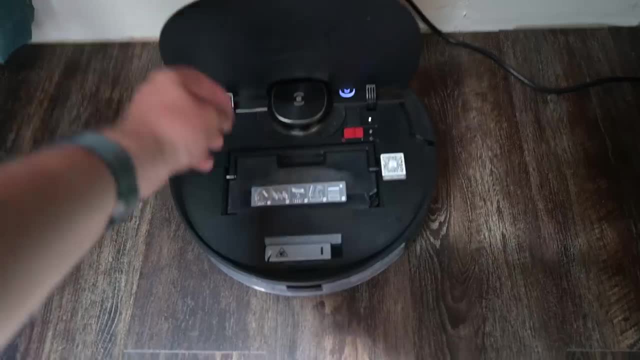 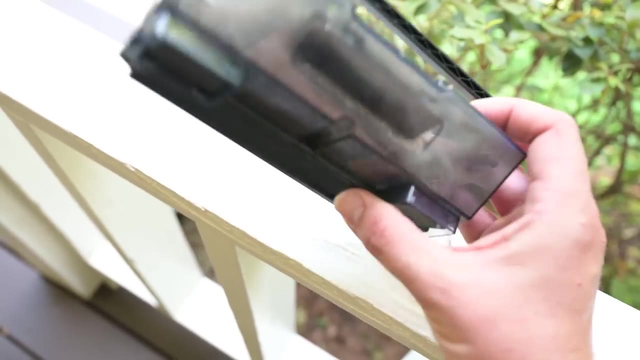 is that I had said in that review that the auto empty bin was not emptying the cat hair from our two cats because the bin was so full of hair that it was getting stuck in the little doors of the bin and that I would try some things over time and report back. Well, after. 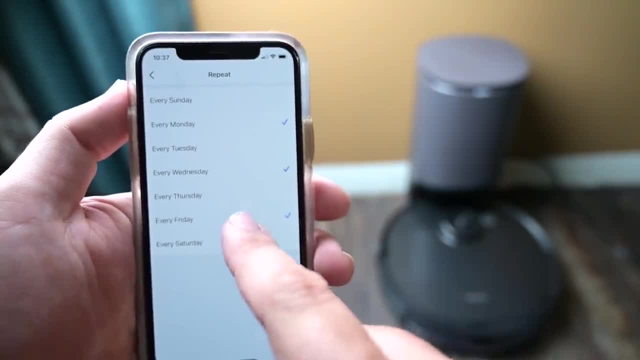 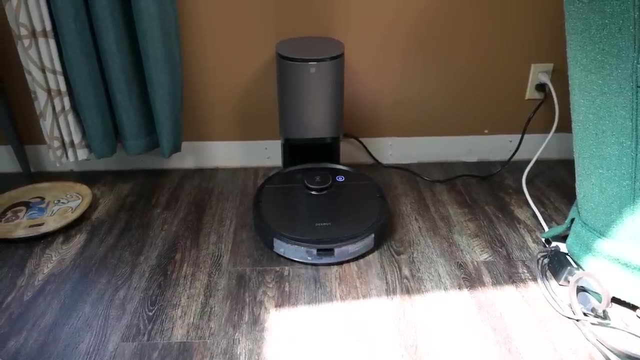 using it regularly, we have found that we have to set the schedule to run three times a week so that the cat hair doesn't build up that much. If we do that, it empties the bin automatically every time, but if it runs any less than three, 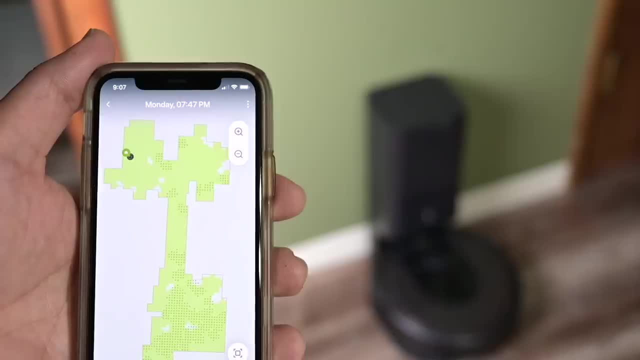 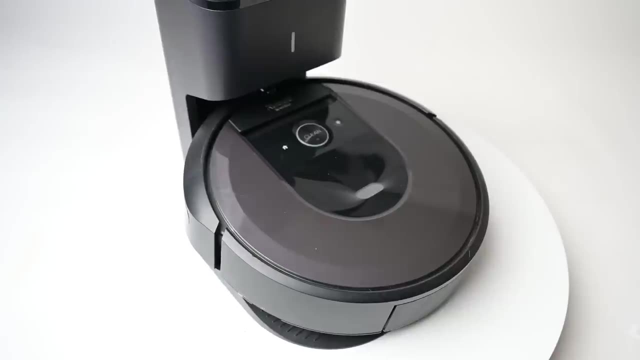 times a week, the hair will get stuck in the bin like before. We've been remodeling our downstairs and have recently started using another auto empty robot vacuum there. In this case it's the iRobot Roomba i7 Plus, which I actually prefer. 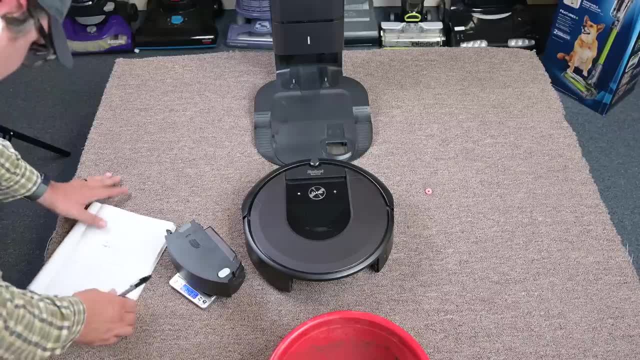 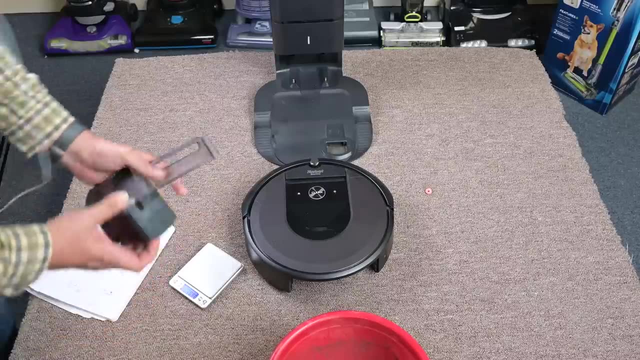 even over the more expensive Roomba S9 Plus. I think I've gotten pretty spoiled by these auto empty bin systems at this point, and iRobot really does make one of the best it comes with. I also like the i7 for our big rug downstairs, because Roombas are just so. 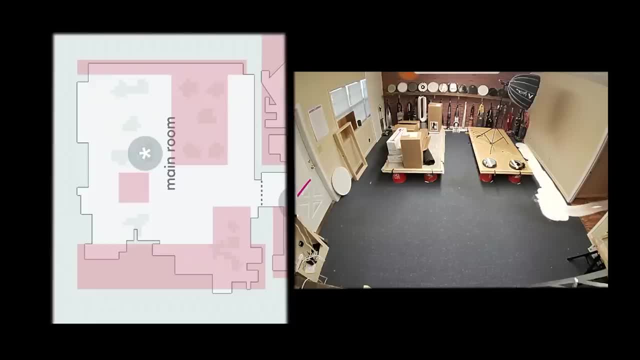 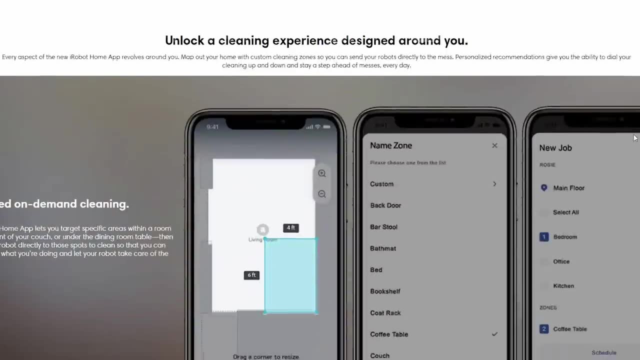 good with deep cleaning carpets. I also wanted something that had app zones, which Roombas do they call them- keep out zones. iRobot has recently updated a lot of things on their app, which we'll talk about in a future video, but the bottom line is that we use the Roomba. i7 Plus downstairs. I run it twice a week with no issues emptying the bin so far. I'm really not sure if that's because the auto empty bin is better than the Acovax with hair or because only one of our cats likes to go downstairs. 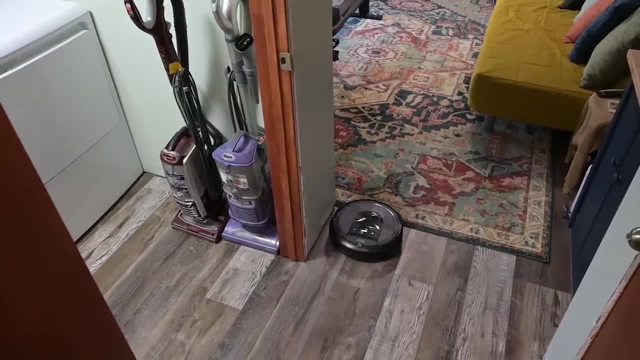 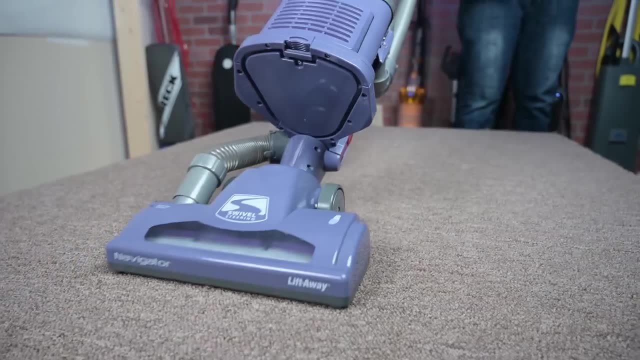 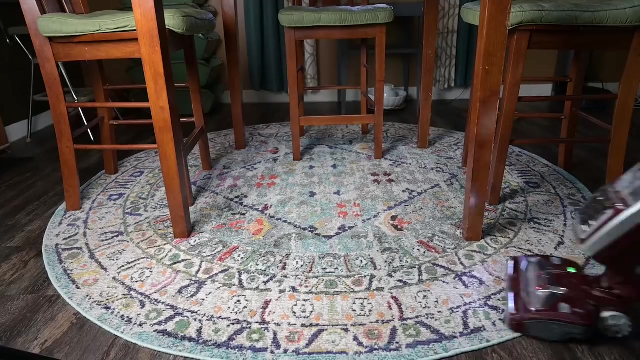 One of the more interesting things I think about this video is that the upright vacuums we use at the house are the same ones we've been using for years: The Shark Navigator Lift Away- NV352 and the Shark Lift Away Speed with Duo Clean- NV803.. These are the ones we